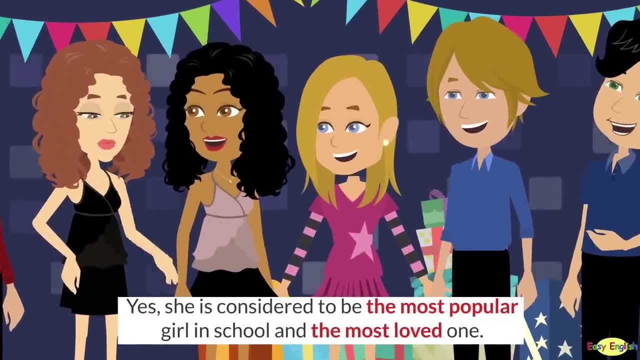 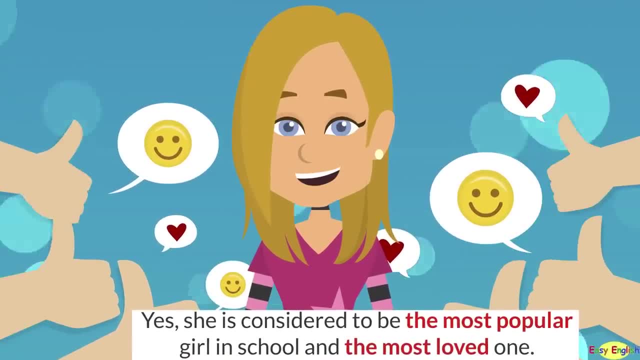 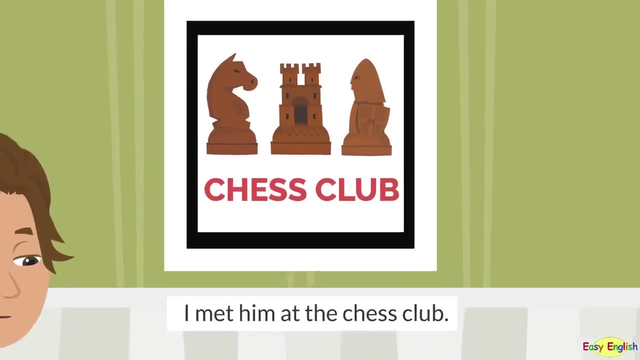 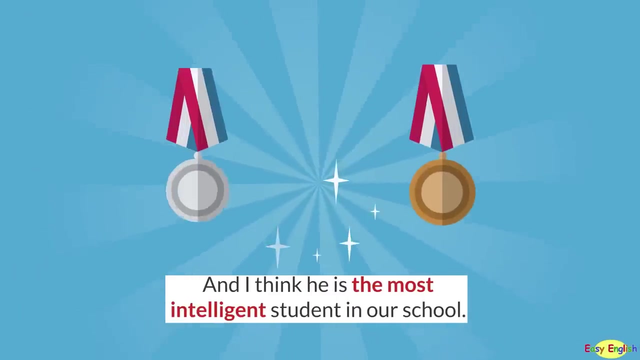 she is. She is considered to be the most popular girl in school and the most loved one. Who is the boy next to her? That's her brother, Paul. I met him at the chess club. He's the most talented chess player in the club And I think he is the most intelligent student in our school. 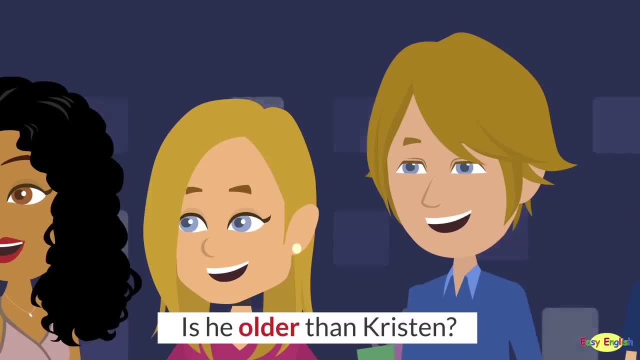 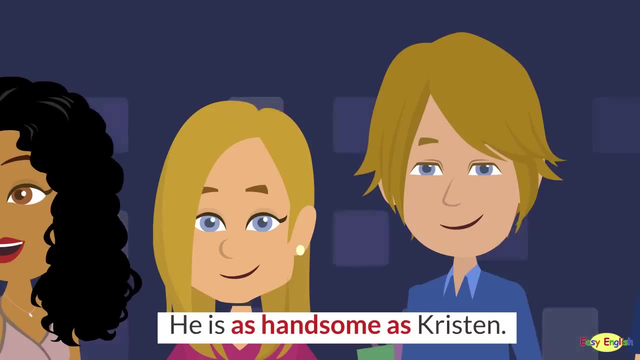 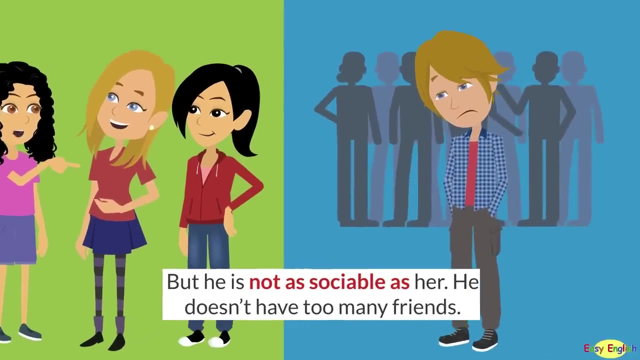 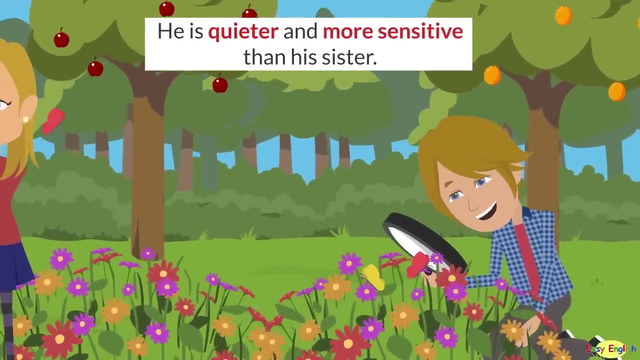 Is he old? Yes he is. Is he older than Kristen? Yes, he is two years older than her. He is as handsome as Kristen, But he is not as sociable as her. He doesn't have too many friends. He is quieter and more sensitive than his sister. He studies harder than her His marks. 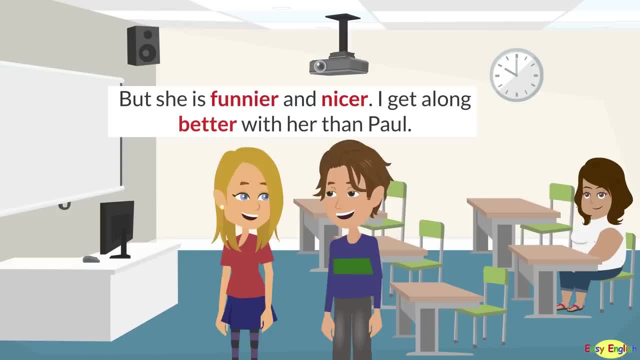 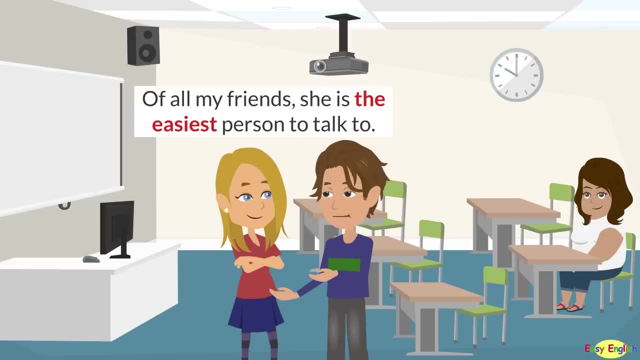 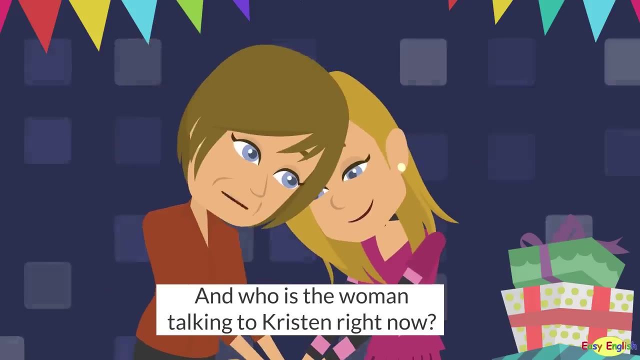 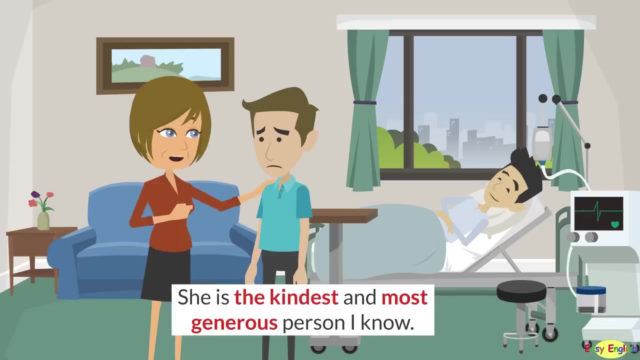 are better than Kristen's, But she is funnier and nicer. I get along better with her than Paul. Of all my friends, she is the easiest person to talk to. And who is the woman talking to Kristen right now? Oh, that's her mum. She is the kindest and most generous person I know. She loves helping. 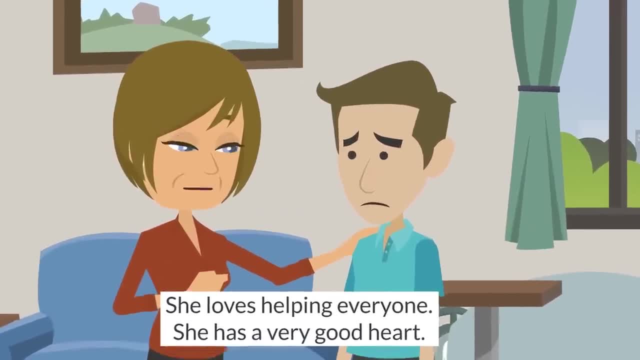 everyone. She has a very good heart and loves to talk about the world with friends. She's very helpful. She will always be there for me and if I need help I will give her my Look. the girl coming towards them is Christian's and Paul's sister, Vivian. 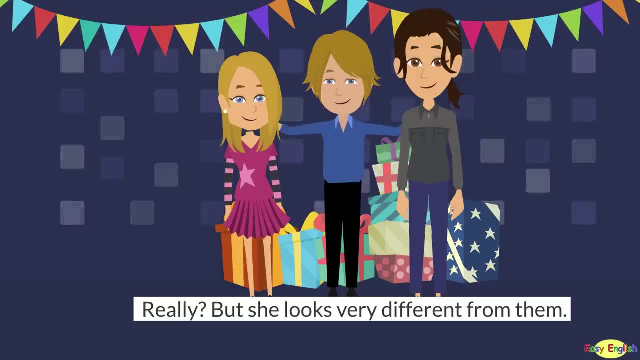 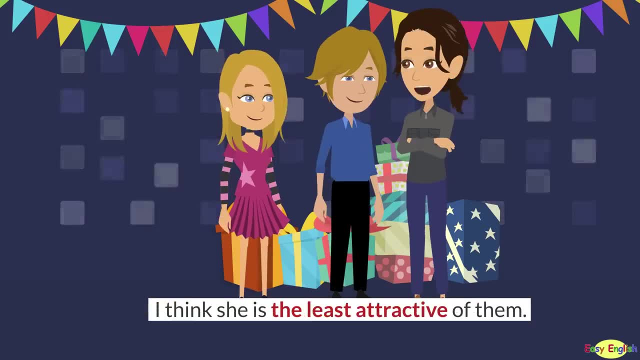 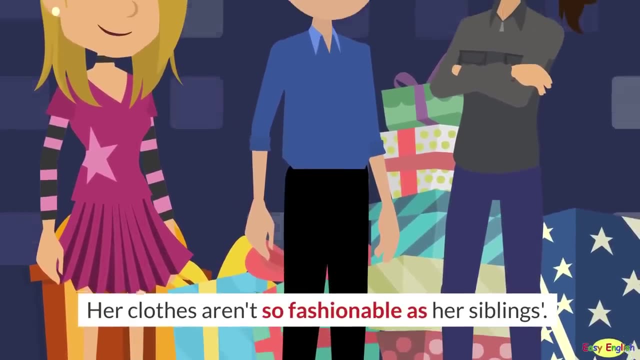 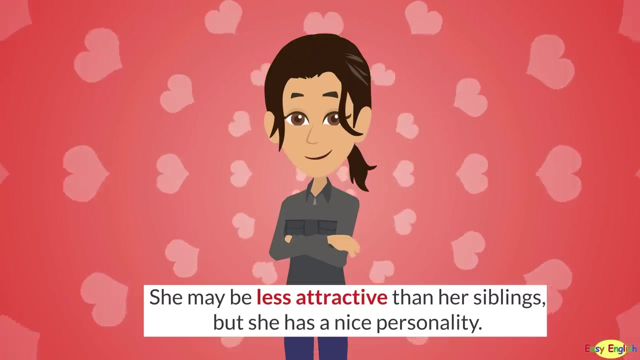 Really. But she looks very different from them. She is taller, has darker hair and looks much older. I think she is the least attractive of them. Her clothes aren't so fashionable as her siblings. Well, I think she considers character more important than appearance. She may be less attractive than her siblings, but she has a nice personality. 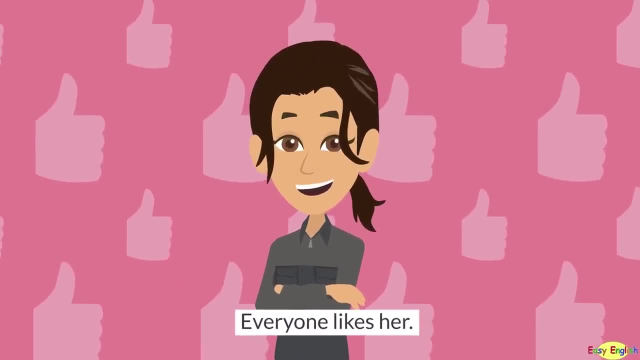 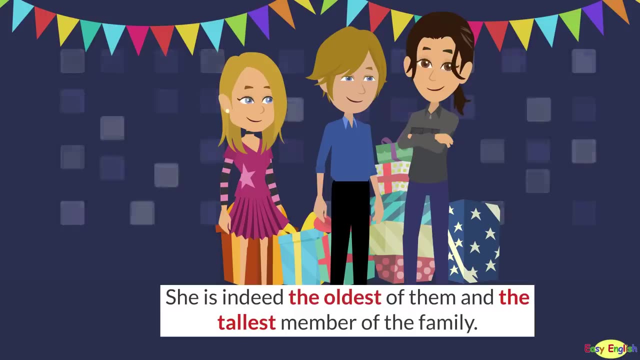 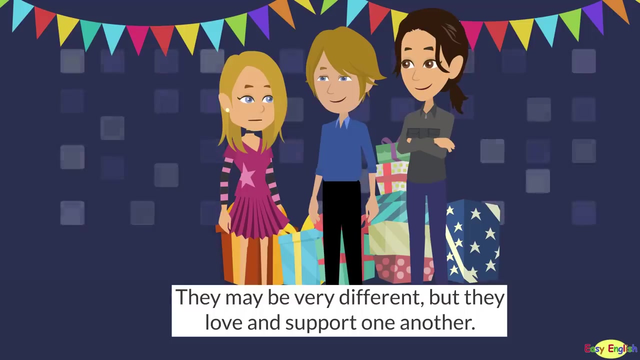 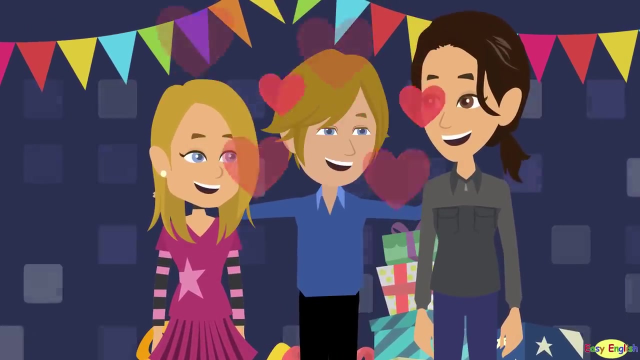 Everyone likes her. She is indeed the oldest of them and the tallest member of the family. She is a basketball player. They may be very different, but they love and support one another. That's the most important thing. How's it going, guys? Are you having fun? 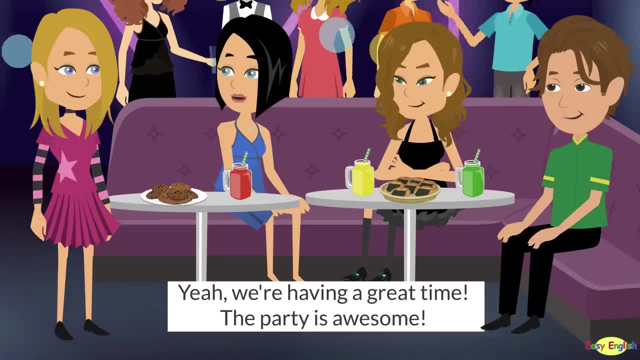 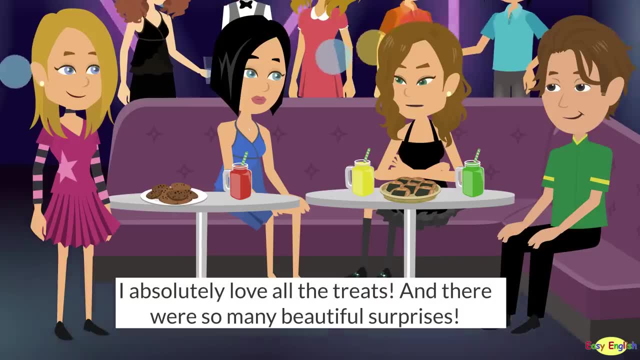 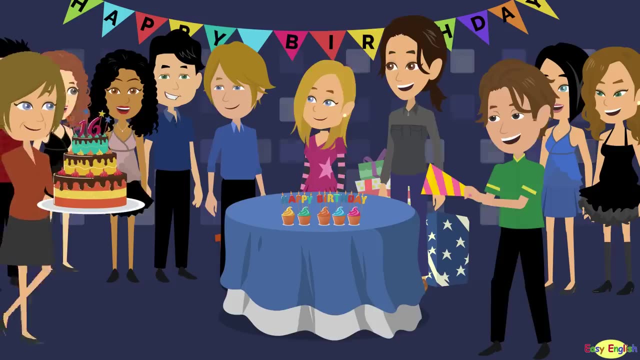 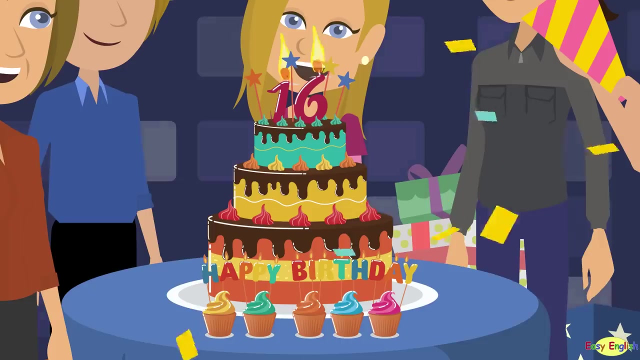 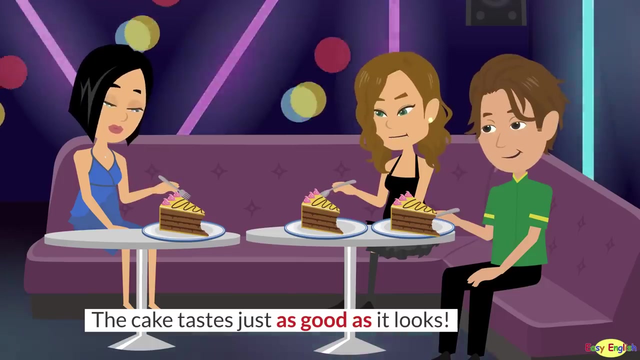 Yeah, we're having a great time. The party is awesome. I absolutely love all the treats And there were so many beautiful surprises. The best part is yet to come. Just wait and see, And with this reward, you're all free to go. Happy Birthday. The cake tastes just as good as it looks. 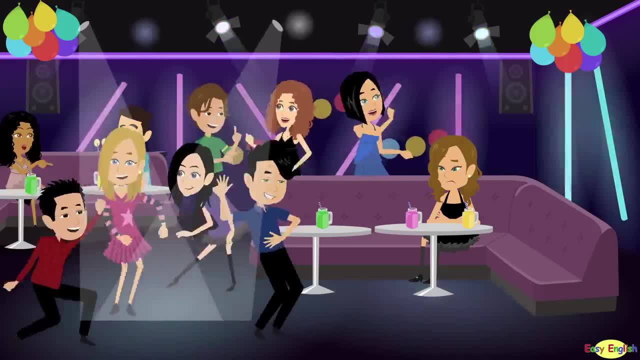 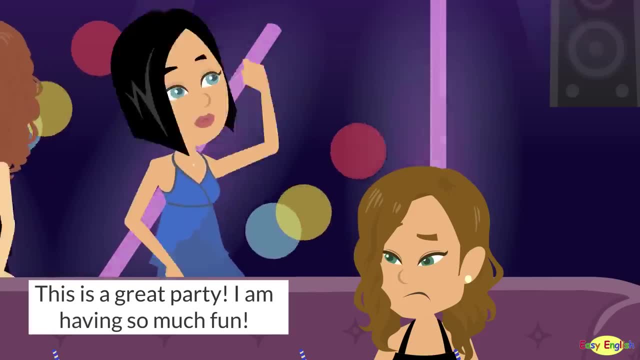 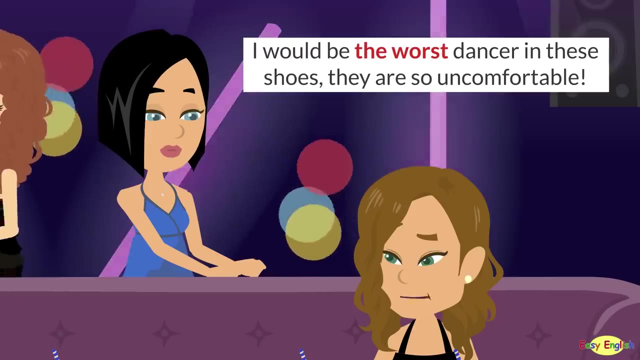 It has the most wonderful flavor I've ever tasted. This is a great party. I am having so much fun. Pam, you are the best dancer in our class. Why won't you join us? would be the worst dancer in these shoes. they're so uncomfortable. so anyone is a. 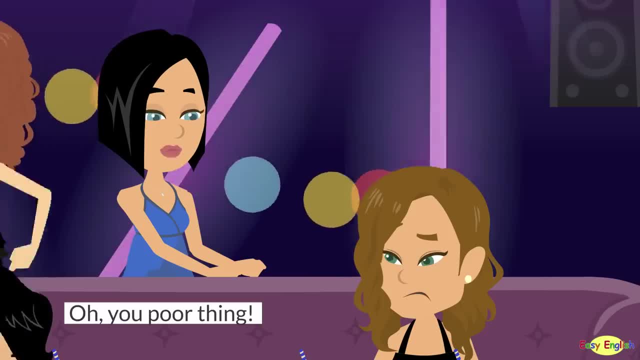 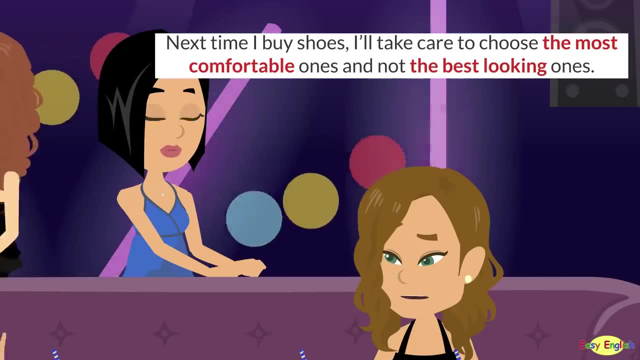 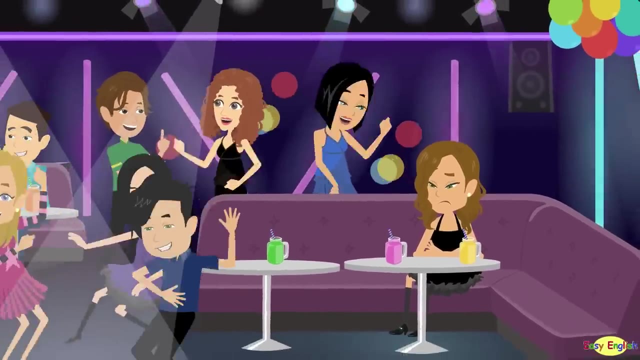 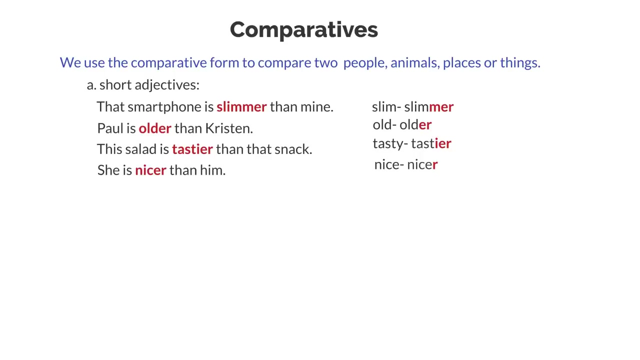 better dancer than I am right now. oh you poor thing. next time I buy shoes, I'll take care to choose the most comfortable ones and not the best-looking ones. comparatives: we use the comparative form to compare two people, animals, places or things. that smartphone is slimmer than mine. 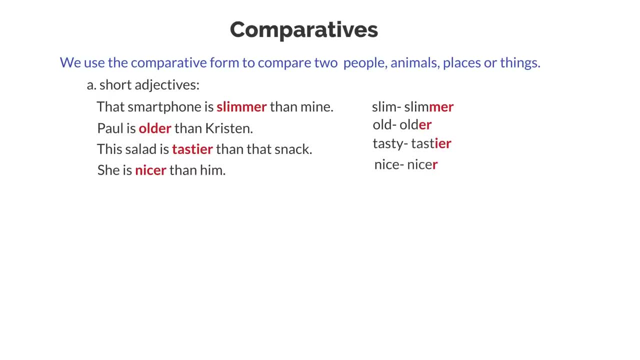 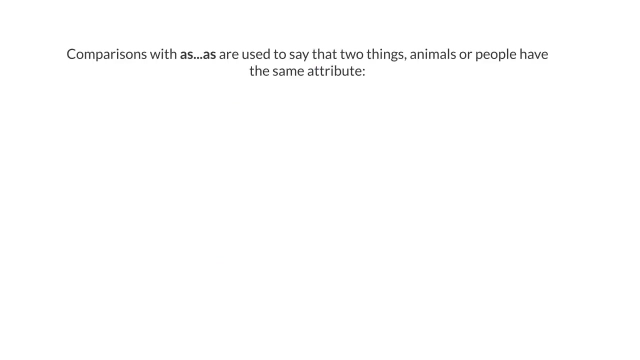 Paul is older than Kristen. this salad is tastier than that snack. she is nicer than him. her phone is more modern than mine. Paul is more sensitive than his sister. you can be on is less attractive than Kristen. you're a better dancer than me. comparisons with SS. or used to say that two things, animals. all people have the. 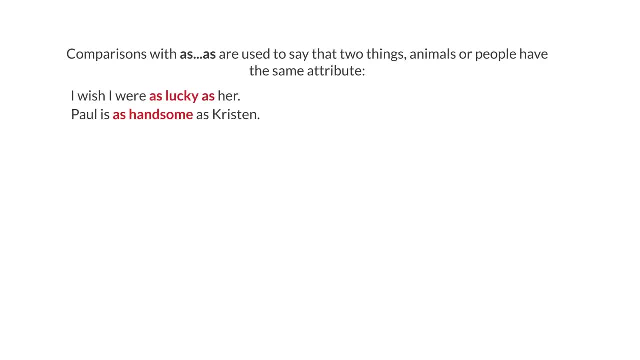 same attribute. I wish I were as lucky as her. Paul is as handsome as Kristen, not as, as is used to say. the two things- animals, all people- do not have the same attribute. not as, as and less have the same meaning. he is not as sociable as her or he is less.